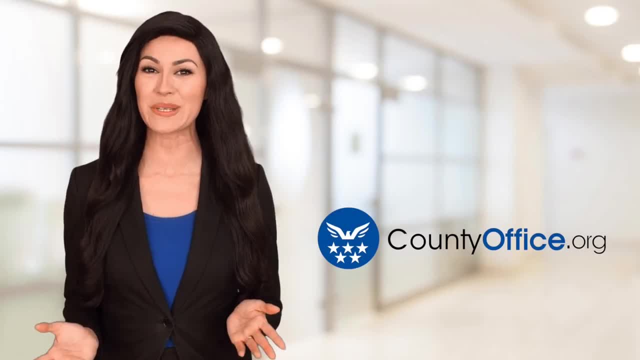 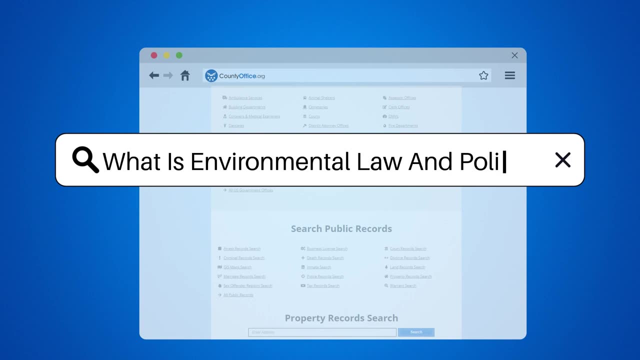 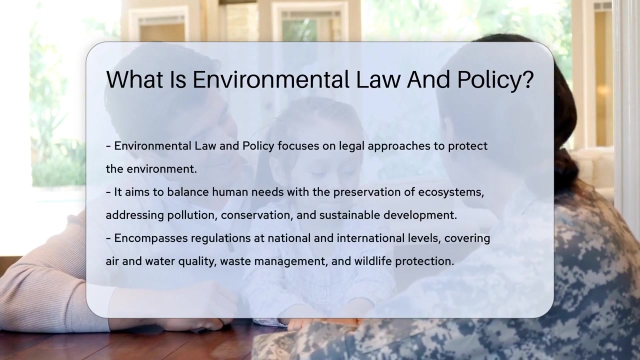 Welcome to County Office, your ultimate guide to local government services and public records. Let's get started. What is environmental law and policy? The realm of environmental law and policy is a complex and dynamic field, focusing on the legal approaches and policies designed to protect the environment. 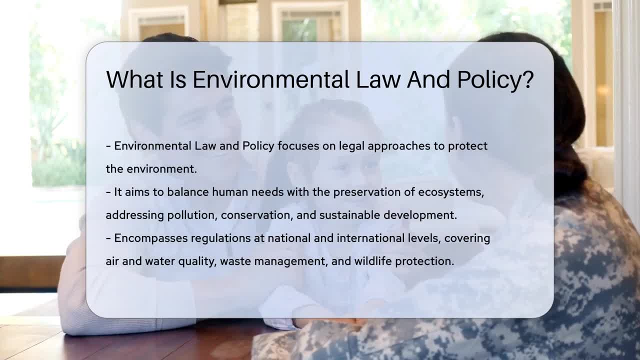 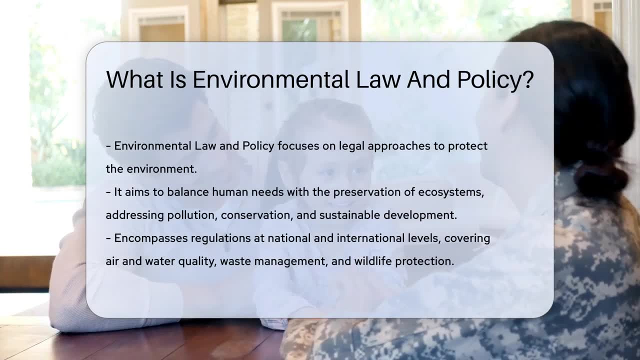 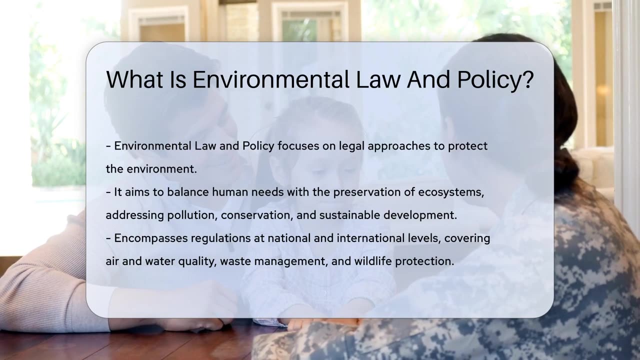 This branch of law seeks to balance human needs with the preservation of natural resources and ecosystems, addressing issues such as pollution conservation and sustainable development. Environmental law encompasses a wide range of regulations and statutes, both at the national and international levels, aimed at controlling activities that impact the environment. 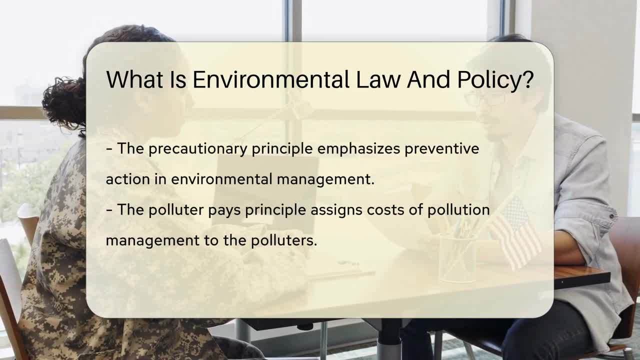 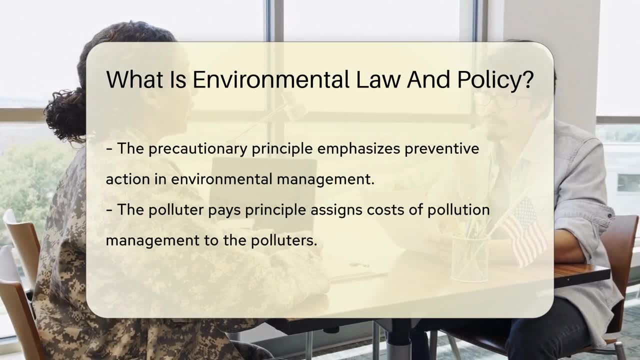 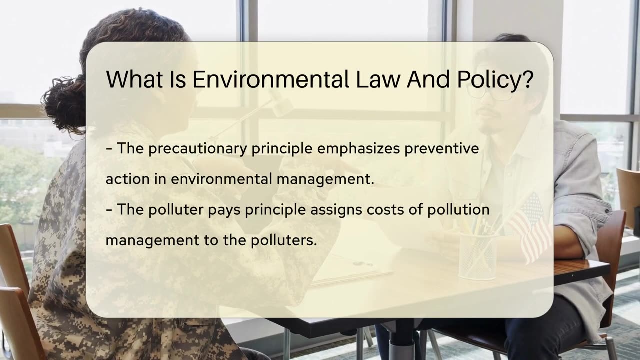 These laws cover various sectors, including air and water quality, waste management and the protection of wildlife and natural habitats. One of the key principles of environmental law is the precautionary principle, which advocates for preventive action in the face of uncertainty regarding potential environmental harm. 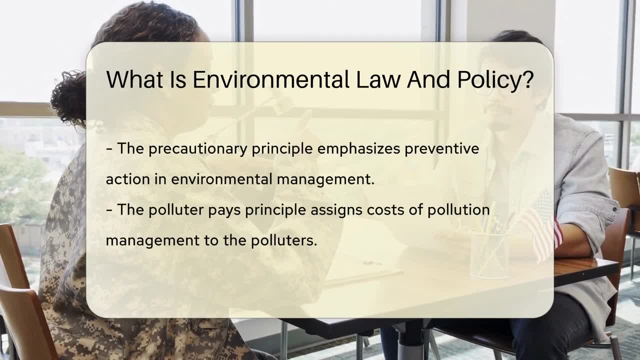 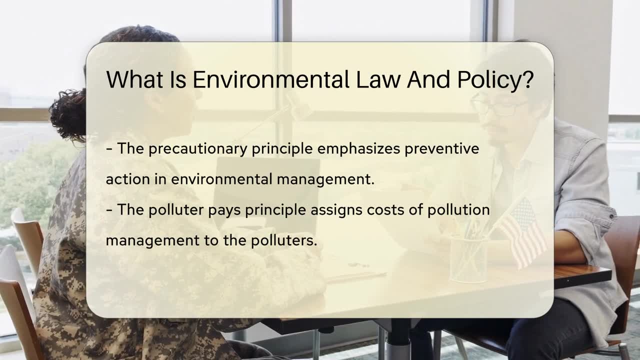 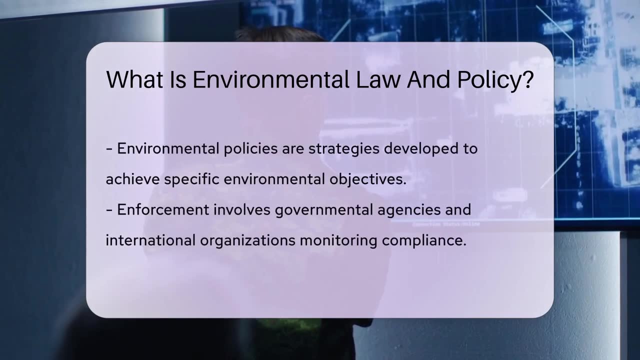 This principle underscores the importance of foresight and prevention in environmental management. Another foundational concept is the polluter pays principle, which holds that those who produce pollution should bear the costs of managing it to prevent damage to human health or the environment. This concept encourages responsible environmental practices among businesses and industries. 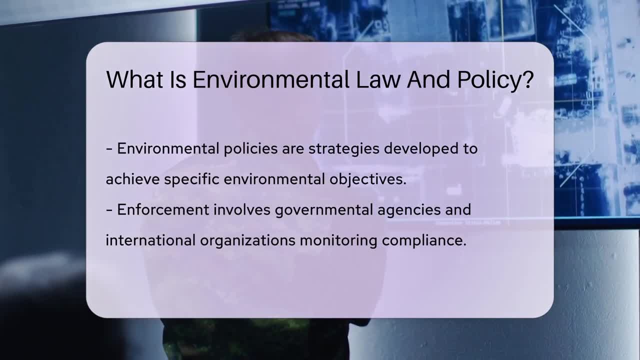 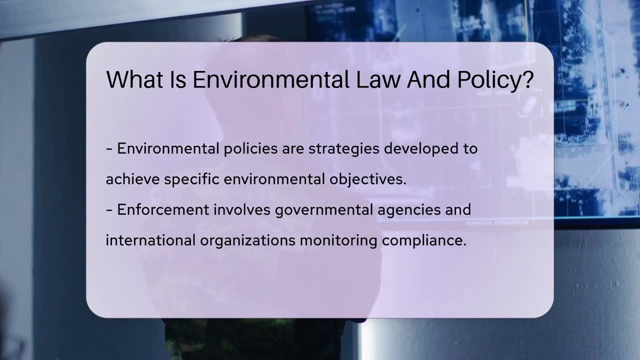 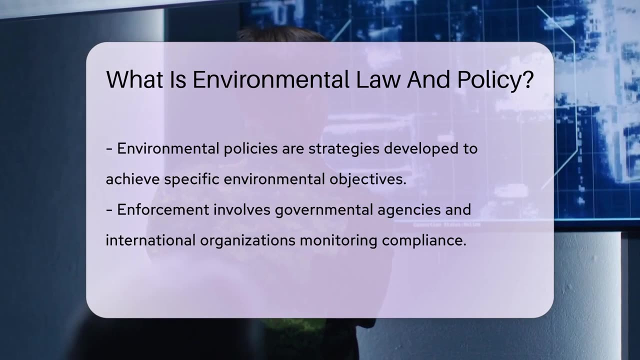 Environmental policies, on the other hand, are strategies and plans developed by governments and organizations to achieve environmental sustainability. These policies guide the implementation of environmental laws and regulations outlining the approaches to be taken in addressing environmental issues. The enforcement of environmental laws and policies involves various governmental agencies. 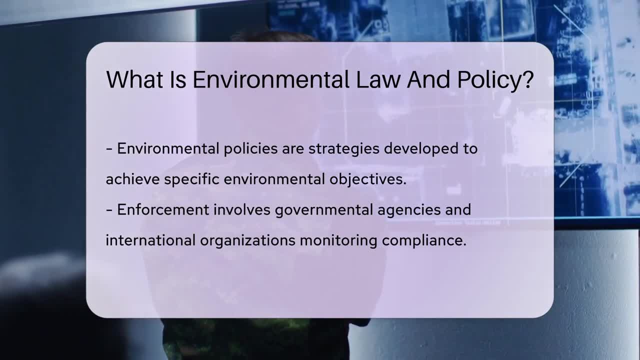 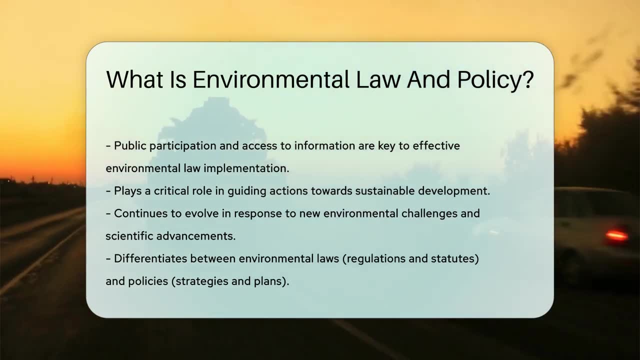 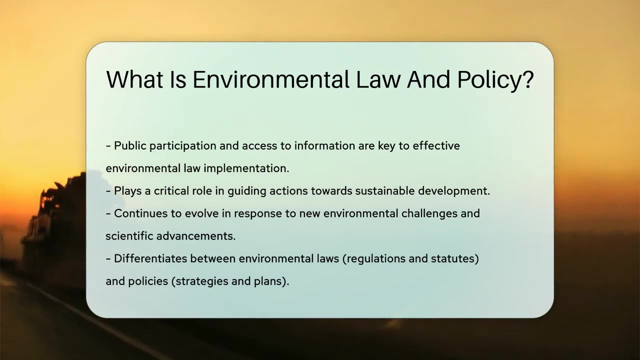 and international organizations which monitor compliance and take action against violations. Public participation and access to information are also integral to the effective implementation of environmental law, empowering individuals and communities to contribute to environmental issues. Environmental law and policy play a critical role in shaping the future of our planet. 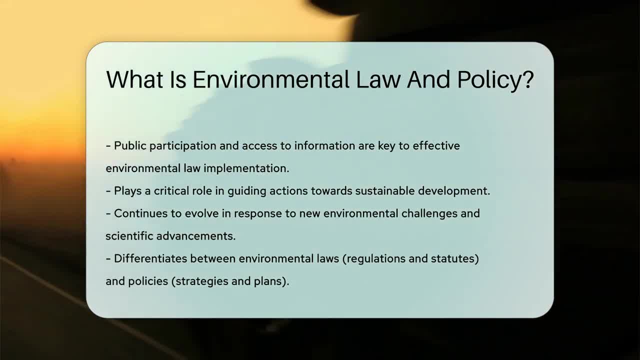 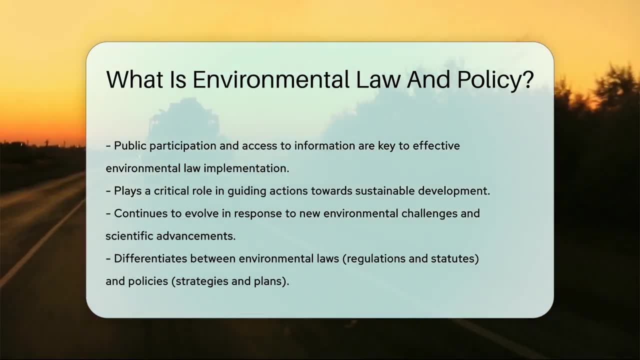 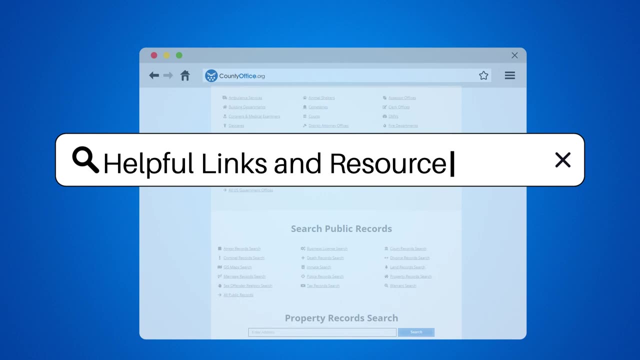 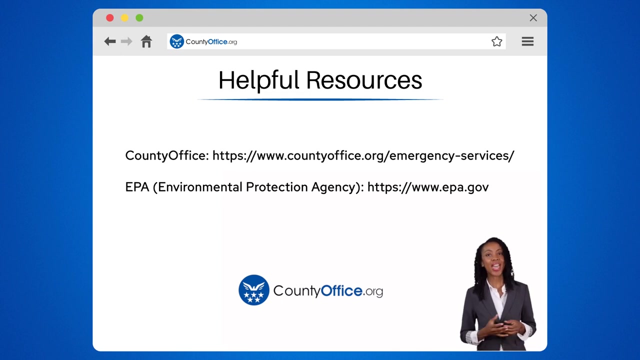 guiding actions toward sustainable development and the conservation of natural resources for future generations. This field continues to evolve in response to emerging environmental challenges and scientific advancements. To learn more, check out these links, which you can click in the description below, And feel free to comment your questions.